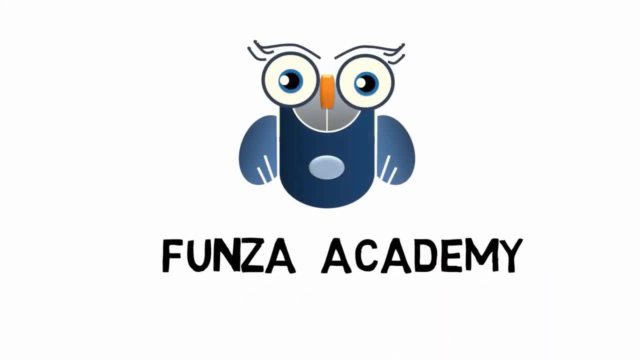 Hello world, and I hope you are doing well in whichever part of the world you are in. Today's problem is a fun little one. The problem involves animals and I want you to firstly visualize the problem and also try to solve it visually. But first, please subscribe to this. 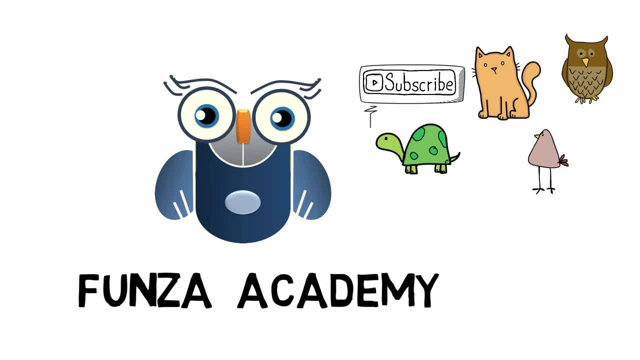 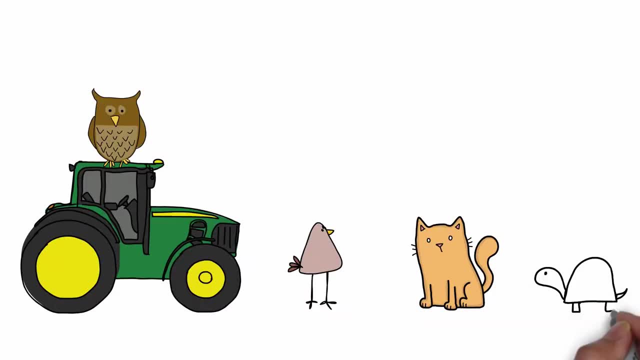 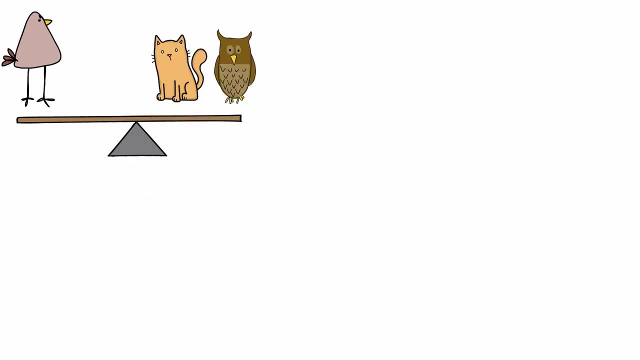 channel We make weekly fun math videos. Thank you, Okay, now here goes So on our animal farm we have four types of animals: Chickens, cats, owls and turtles. One chicken weighs as much as one cat and one owl- Yes, it's a super chicken. Two chickens weigh as much as three turtles. and finally, one owl and one turtle weigh the same as one cat. Now, given this information, the question for you is: how many owls weigh as much as one cat? Please pause the video and get back to the video. Please subscribe to this channel. Thank you, Bye, bye. 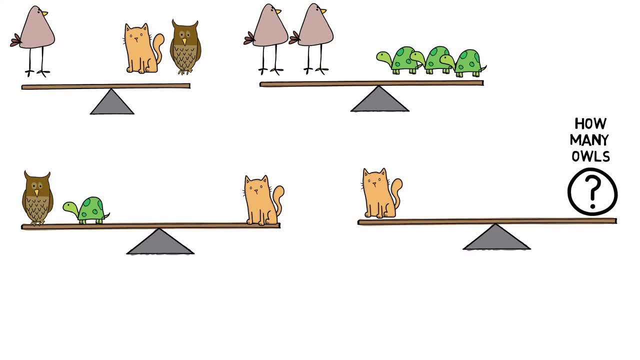 Give the problem a try and, when finished, do come back and keep watching. Welcome back Now. I'm going to solve this problem visually. So let us first see what we have On our animal farm. we have chickens, cats, owls and turtles. And now let's focus on what we want. 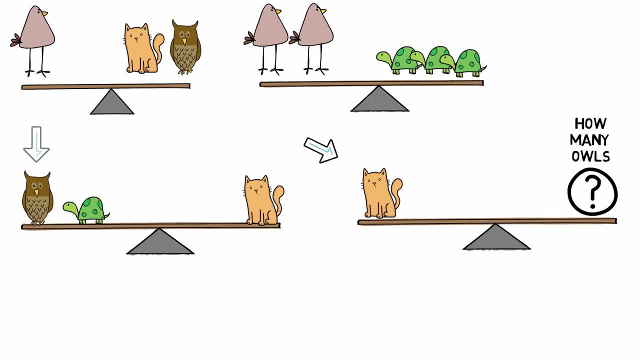 We want the relationship between a cat and an owl. Oops, Relationship may not be the best word here, and don't get me wrong, But what we want to know is how many owls balance one cat in weight? So we are looking at two animals in our answer: Owl and cat. So let's 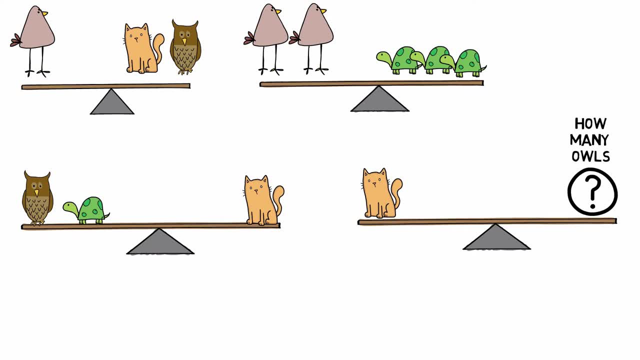 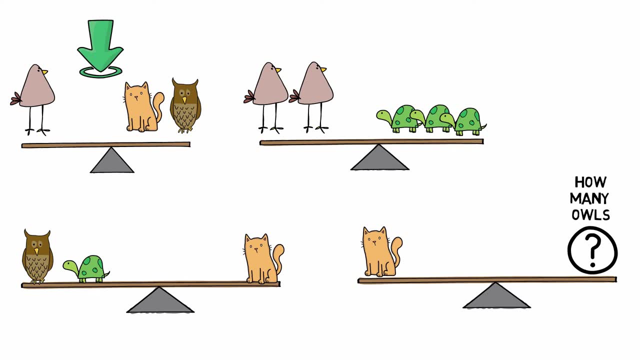 try to get to these two animals Now. from this first figure we know that one chicken is equal to one cat and one owl in weight. Now, in the answer we are looking for, we do not need a chicken, so let's try to get rid of it Now. if one chicken weighs the same as one cat and one owl, we can say: 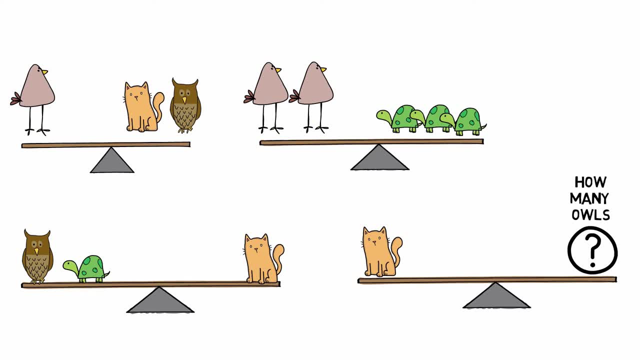 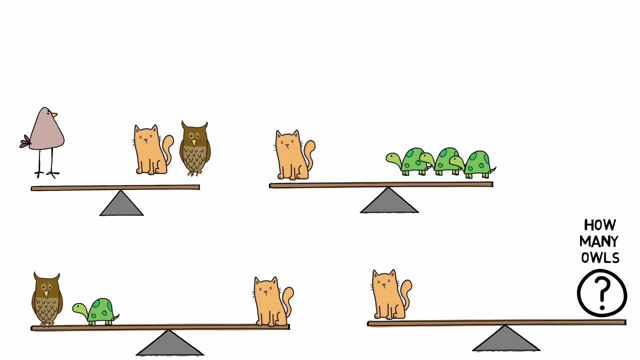 that two chickens weigh as much as one owl. We can say that two chickens weigh as much as one owl, as two cats and two owls, And we will use this information here. So let's replace the two chickens with two cats and two owls, So we have two cats and two owls weigh as much as three turtles. 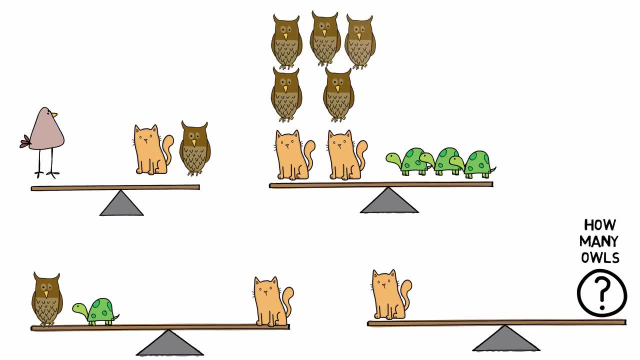 Now pay attention to this interesting step. I'm going to add three owls to both sides. Doing so does not make a difference, since the three owls will balance each other out Right. So now we have five owls is equal to three owls and three turtles. So how does this help us? As per this figure one,